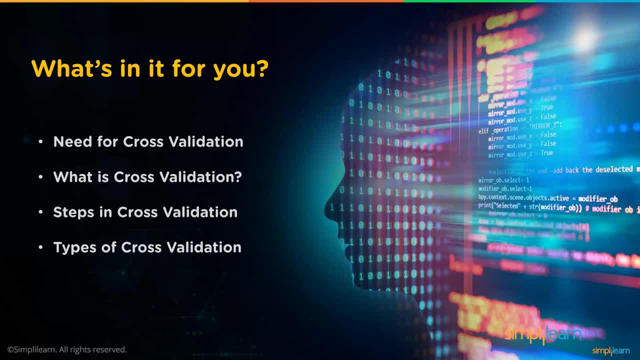 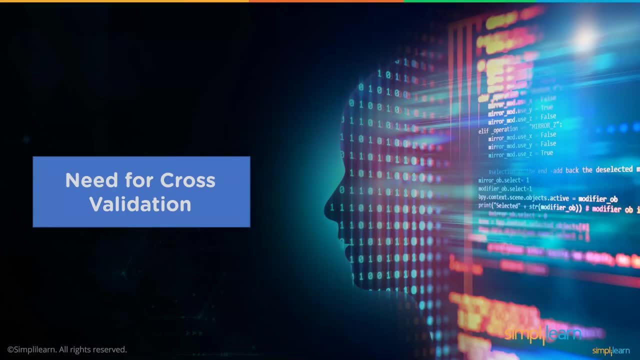 and types of cross-validation, And then, of course, we'll do a nice hands-on demo so you can see what it looks like in Python code. Let's start by exploring the need for cross-validation While choosing machine learning models. we need to compare models to see how different models 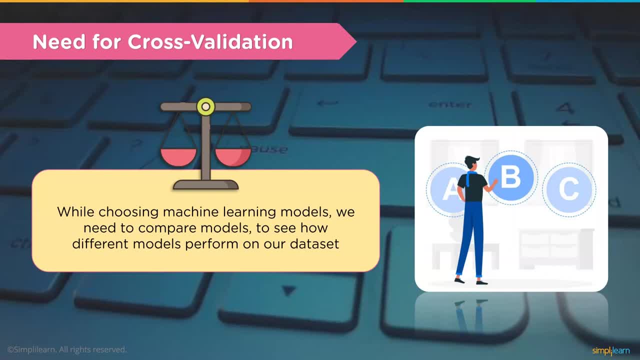 perform on our data set. This goes beyond just comparing different models, but also in explaining this to the shareholders or whoever you're working with, You really need to know how valid is your data set or your models that you're working with on the data set. So the need for 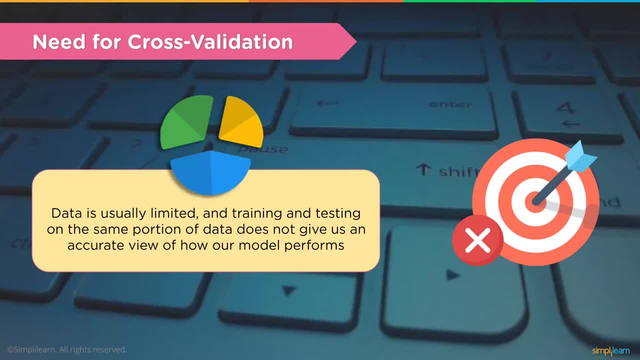 cross-validation comes up when the data is usually limited and training and testing on the same portion of data does not give us an accurate view of how our model performs. And this just makes sense. If I'm going to program a model to out guess something, I don't want to use the same. 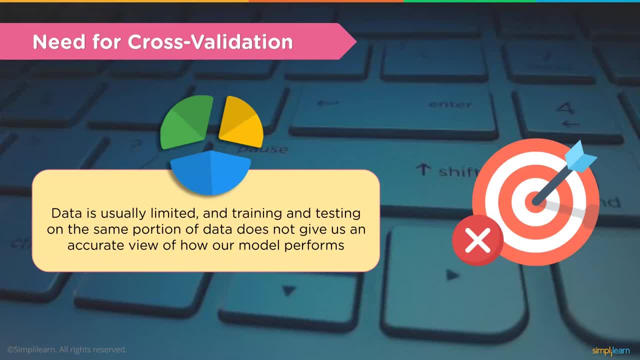 data I trained it with. I want to see how it performs on the next data. Otherwise, I'm just giving myself my own juice saying, hey, my model did really good, because this is what it was based on- Self-fulfilling prophecy- And that is still important to do because you still need to run it. 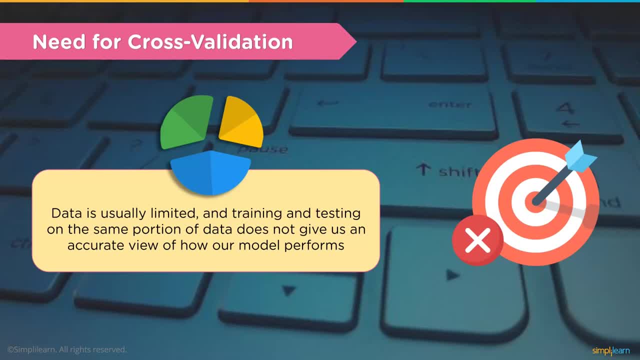 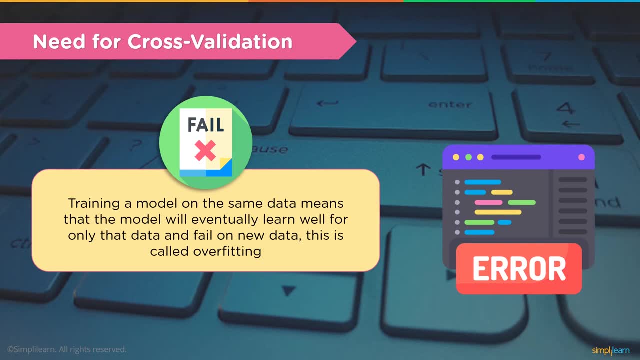 on your own data to see how well your set fits your data versus how well it fits new data coming in. So training a model on the same data means that the model will eventually learn well for only that data and fail on new data. This is called overfitting. So you might write a wonderful 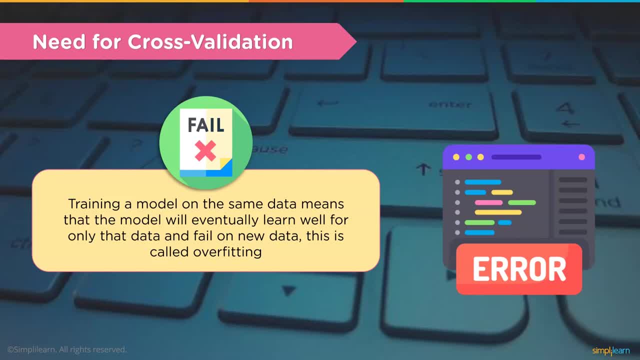 script. It works great, but it's not going to work. So you might write a wonderful script. It works great, but it's not going to work. So you might write a wonderful script. It works great for predicting the failure on loans for a bank, but it only works for the data you already have. 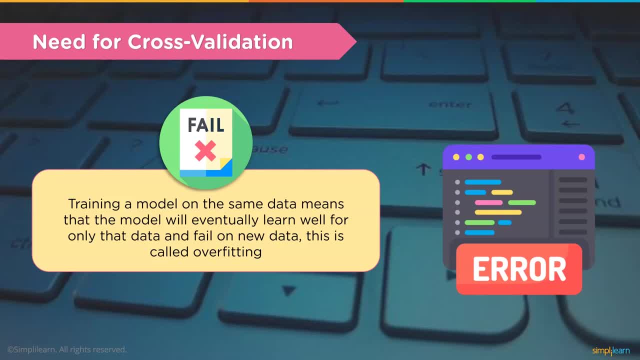 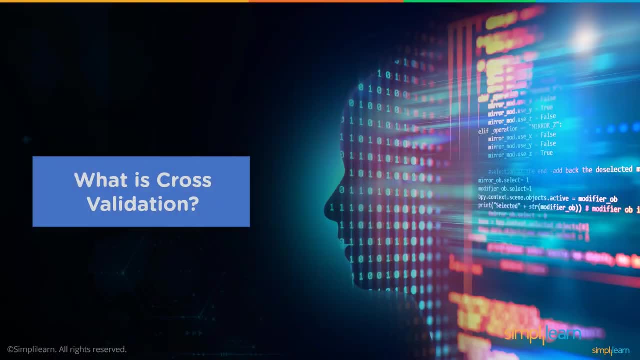 not the new data coming in And that again is overfitting. So it's not going to give you a proper. you're not going to get a good value as to how good your model is going to fit the new data coming in. So what is cross-validation? Cross-validation is a technique which is used to 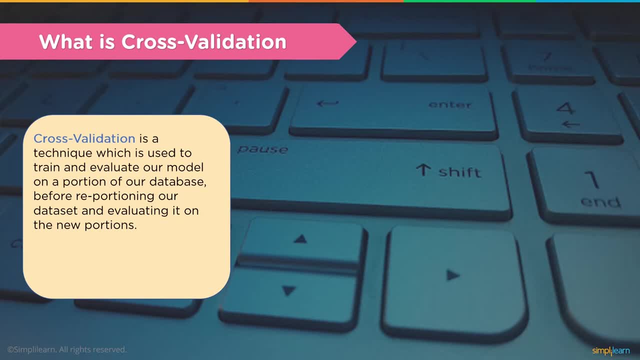 train and evaluate our model on a portion of our database before reportioning our data set and eventually using it on the new portions. So what is cross-validation? Cross-validation is a technique which is used to train and evaluate our model on a portion of our database before reportioning our data set and eventually using it on the new portions. 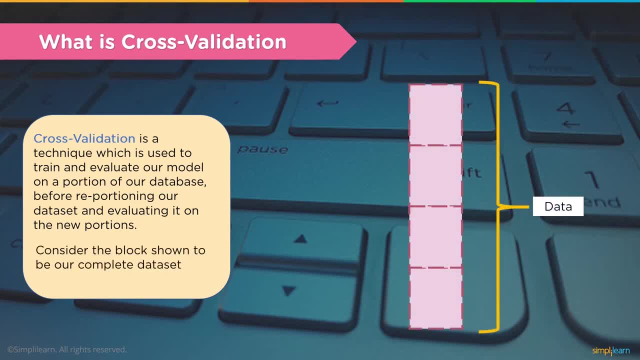 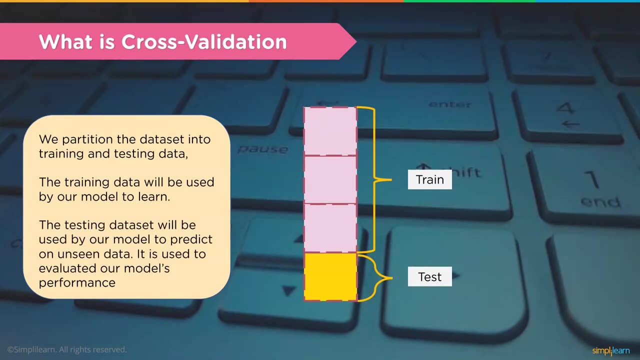 Consider the block shown to be our complete data set And you can see we've already taken the data set and divided it into four sections, And here we've cut out one section highlighted in yellow. We partition the data set into training and testing data And you'll see that in this. 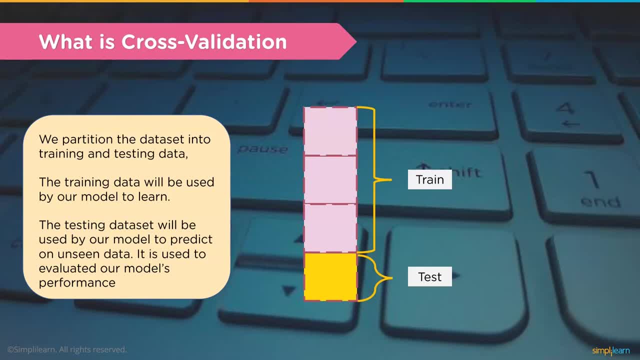 particular example, we've taken 75 percent of the data, or three-quarters of it, and we said: okay, we're going to use that to train our model And the testing data set will be used to train, used by our model to predict on unseen data. it is used to evaluate our models. 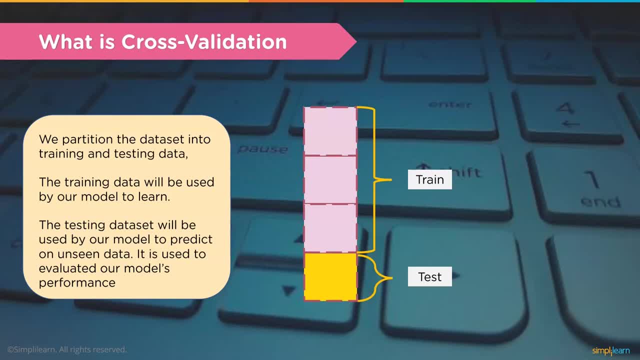 performance, and this is what we're talking about- is you want to be able to train it on one set of data. come back and say, hey, this is how well performs on data. it's never seen before. now there's an interesting relationship between these and it's important to also see how well it performs on the train data we're. 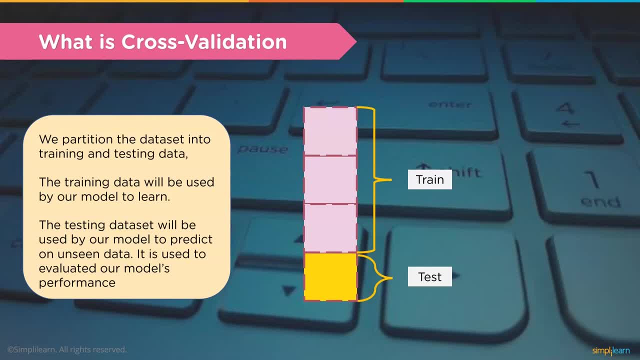 not going to talk about too much on that. one is usually used in higher-end neural networks and it's one of the ways they know when the training data is done and the testing data and the predictions kind of match. that's when they start looking at: okay, you've trained it enough. 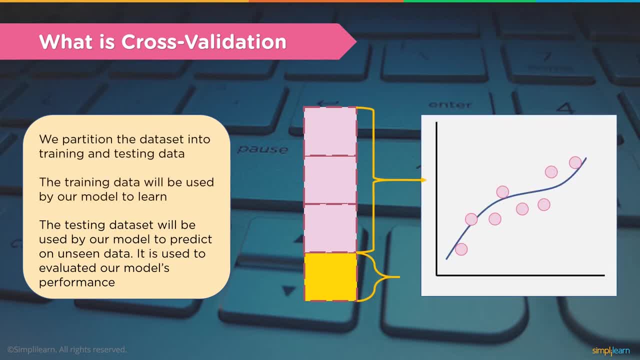 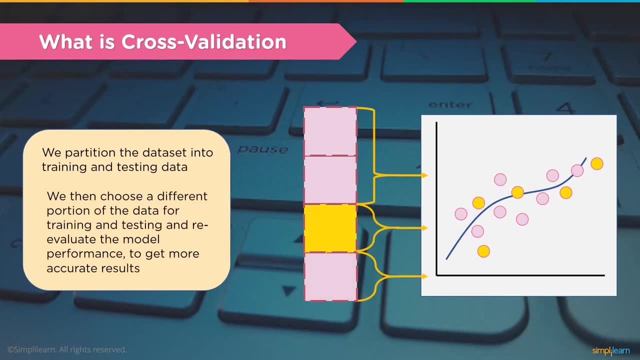 and you can see here we take the first partition in, we go ahead and we map how good it did and we partition the dataset into training and testing data. we then choose a different portion of the data for training and testing and reevaluate the model performance to get more accurate results. And you can see here we've 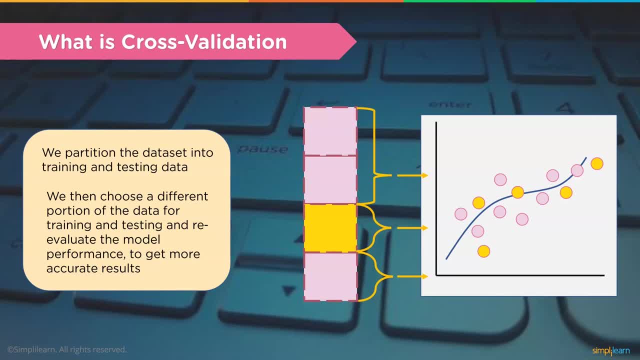 colored it in a nice, pretty yellow for you, And so we've tested on the first section and now we're testing it on the second section. So we're still using three quarters of the data to train our model and one quarter to test it, And we just loop through all the different quarters to test it. 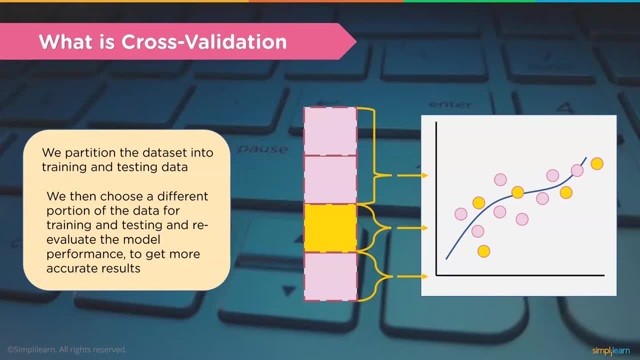 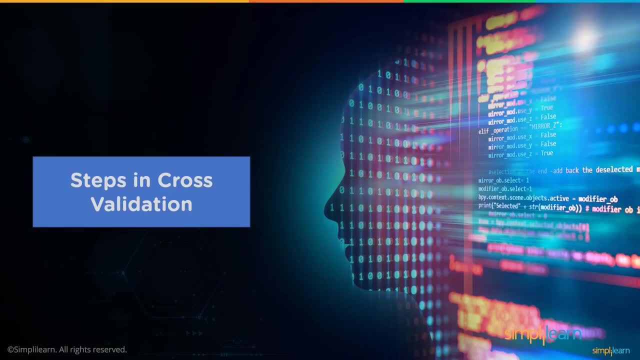 That's what we're talking about when we talk about cross-validation is we want to be able to get a picture of how it works on the data it hasn't seen And we look at the steps in cross-validation. The steps involved in cross-validation begin with step one: split the. 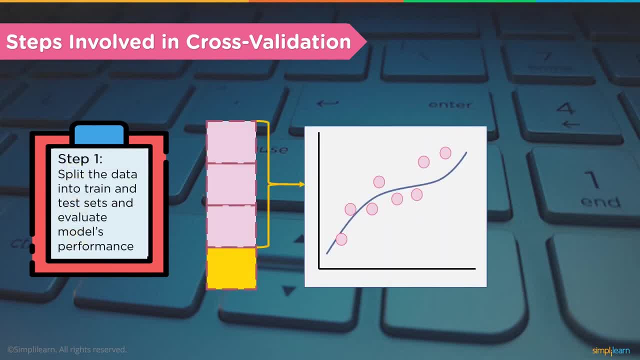 data into train and test sets and evaluate model's performance. And so we measure one, we measure two, we measure three and we measure four, And each one of these generates its own performance rate based on the other 75 percent being used. 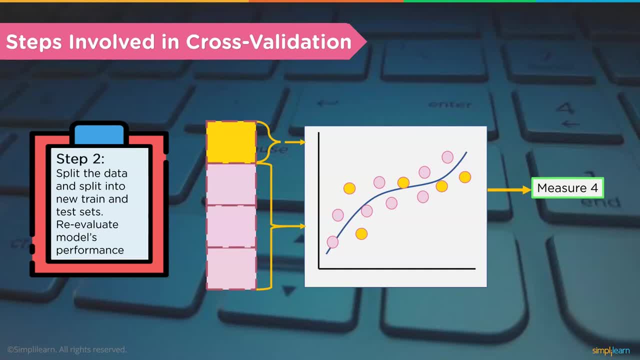 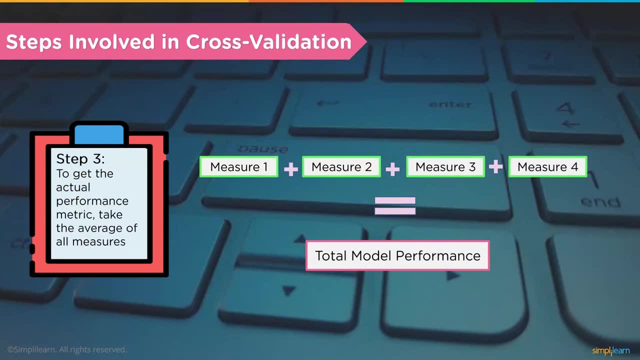 and the other 75 percent being used to validate that data. How well does it perform on the unseen data? And so we have actually created four separate models, And then we just take those measurements- one, two, three, four, we add them together. 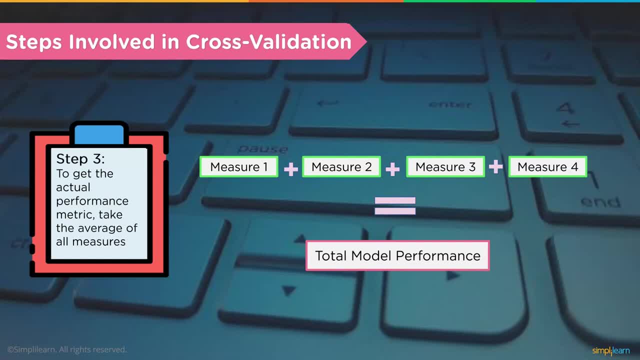 divide by four or however many divisions you use, and you get a total model performance. For myself, when I first start doing a new data set, I'll start with just partitioning it into three, because it runs faster, it's quick. 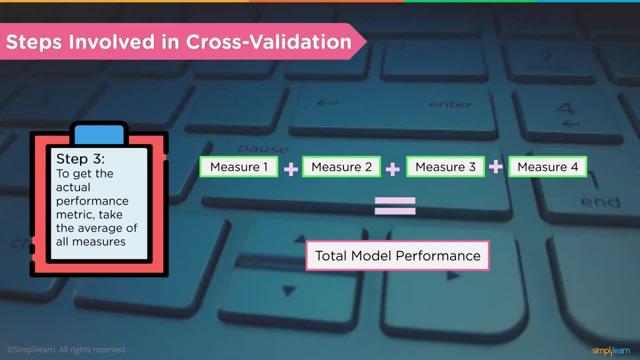 You only have to run three models, that kind of setup. A lot of this depends on how much data you have. If you have a lot of data, three works just fine. If you're very limited on how much data is coming in, you might want to divide it into. 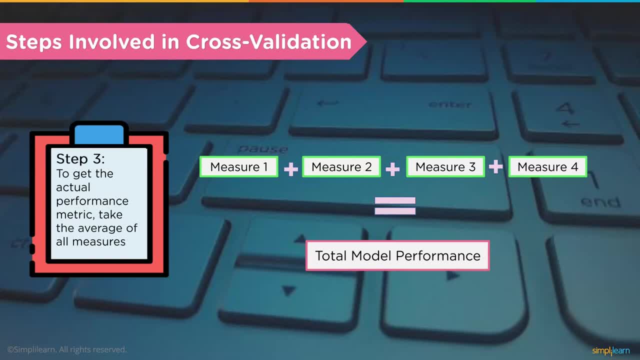 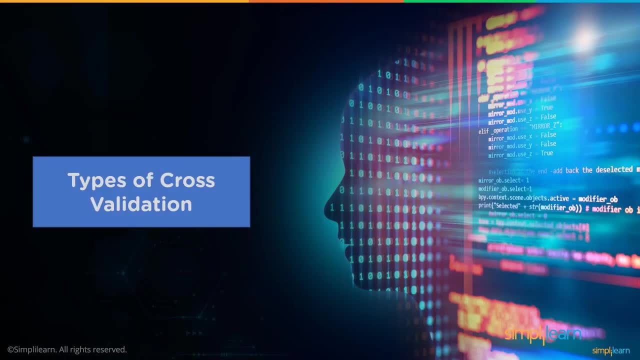 more validation sets when you're first testing out your models and your data sets. And there's other steps in here we'll look at in just a moment Types of cross-validation. Now, this is important because we looked at one type. This is actually what we're going to put down as the number two type. 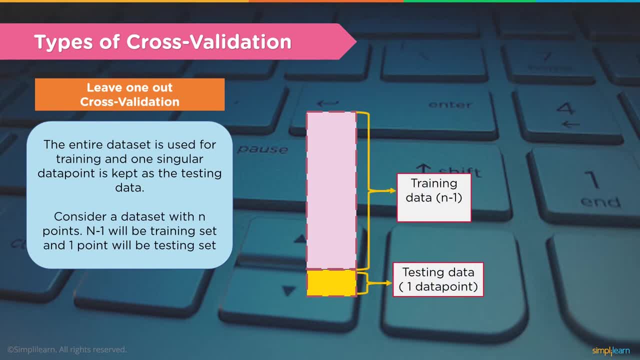 One of the ways we can do this is what they call leave-one-out cross-validation. This is where the entire data set is used for training and one singular data point is kept as the testing data. Consider a data set with n points: n-1 will be training set and one point will be testing set- Leave-one-out. 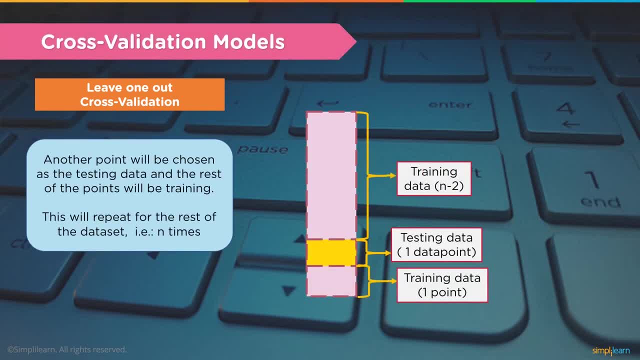 cross-validation is. then we go to another point and it'll be chosen as a testing data and the rest of the points will be the training. This will repeat for the rest of the data. set n times. And yes, we're creating. if your data is n. 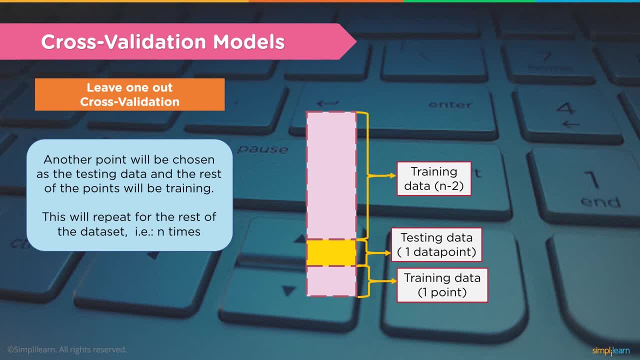 well, they used n-1n, so we'll do it n-1 times and you create n-1 models that you're testing across your data set to see how good your model does. The final performance measure will be the average of the measures for all n. 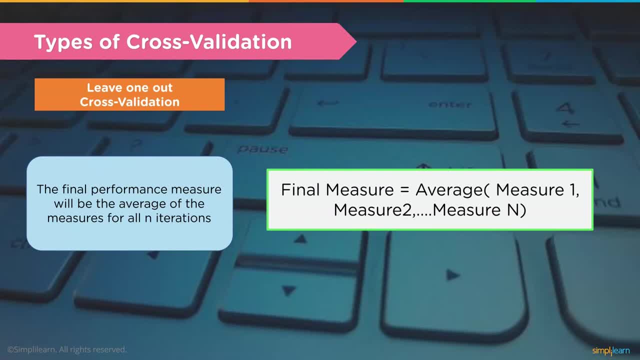 iterations, And so you add up all those different measures and divide by n-1.. Now, keep in mind, at the end you just run it across, all the data and that's your final model that you're going to actually push out. 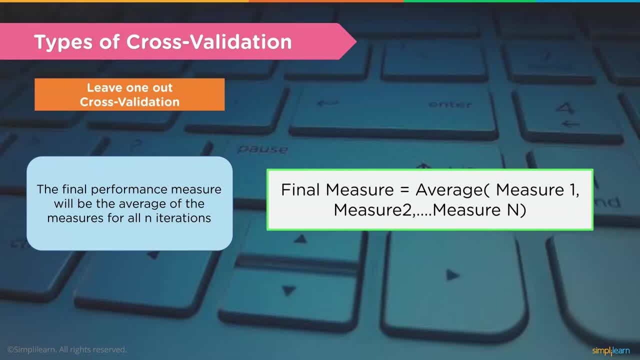 This is to validate it. This gives it an n-1 validation. You can imagine if you're dealing with big data and you have terabytes of data. doing it this way would probably be a very bad idea. You might have to wait a month before you. 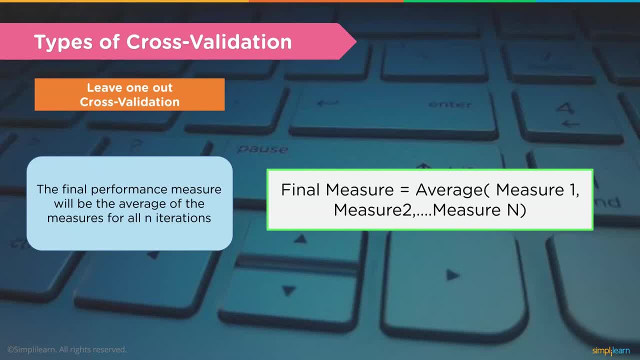 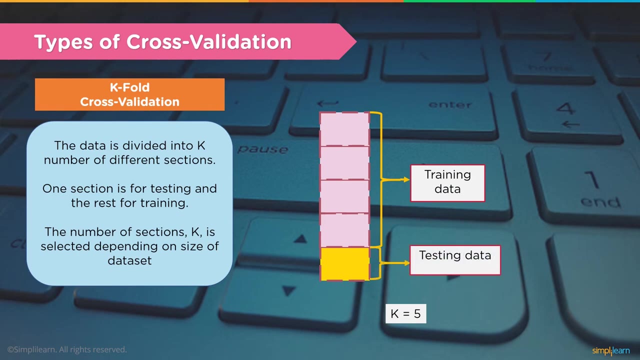 get an answer Where dividing it into smaller portion works. So again, we're dealing with smaller amounts of data. usually when you do this level of cross-validation- k-fold cross-validation. This is what our example initially was and this is what most people look at as you divide it into, in this case, four sections. So 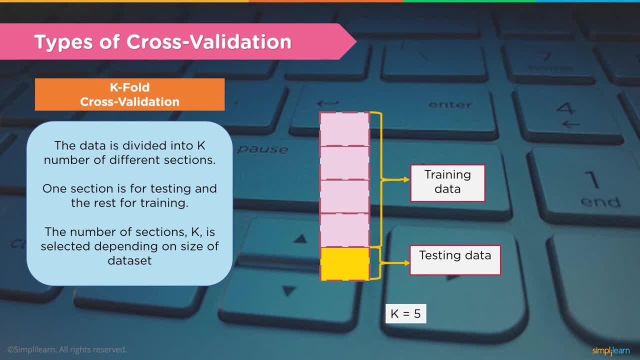 the data is divided into k number of different sections. Like I said, I like to use three. if I'm just initially looking at the data, It gives a decent training model versus a faster run. So at least I know I'm using 66.66% of the data. One. 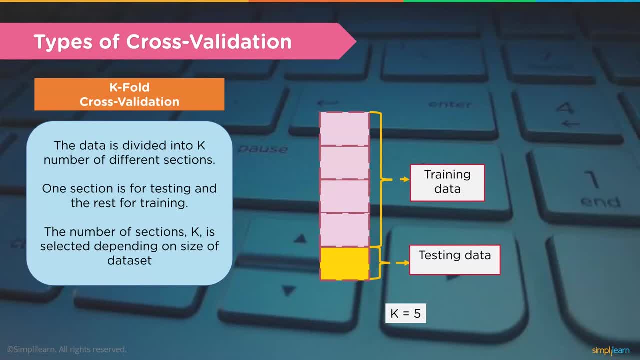 section is for testing and the rest for training. The number of sections, k, is selected depending on certain numbers. So that's about it for this video. So thank you and have a great day. size of data set. Again, if you have a very small data set, you want your k to be much larger. 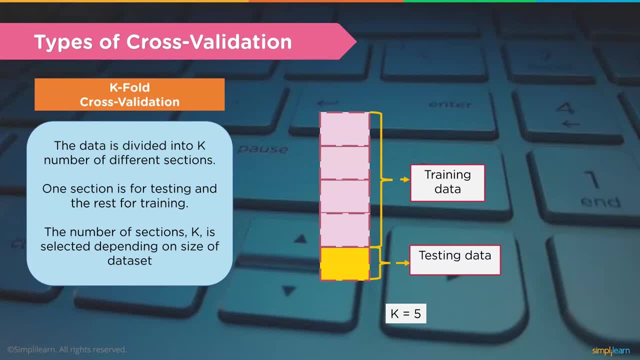 because you- just you- really can't divide out most of your data. You lose so much in the training and so if you divide it out enough, you end up with leave one out. cross-validation: We divide it all the way to. each data point gets its own run and this will generate, if we do k, k equals. 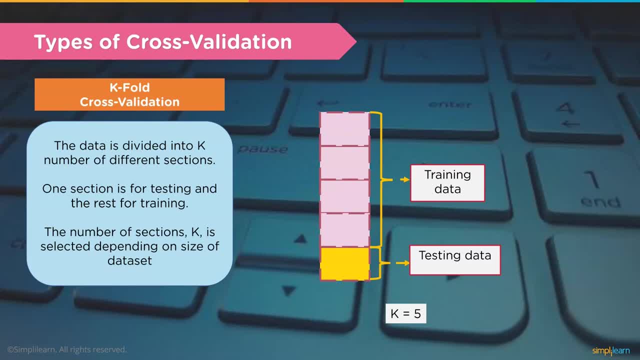 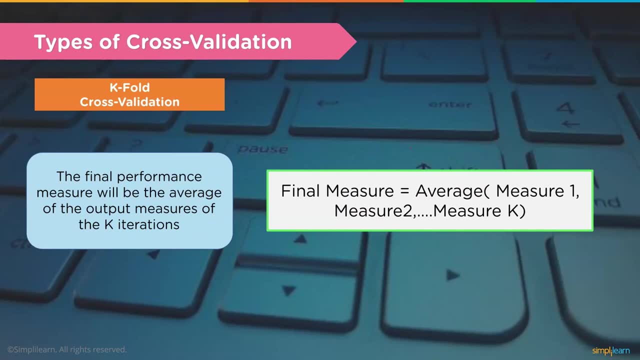 five. it will generate five different models for you to evaluate on, and so, of course, we're generating each one. The final performance measure will be the average of the output measures of the k iterations. so we add them all together and we divide by k. so we're going to have five models. 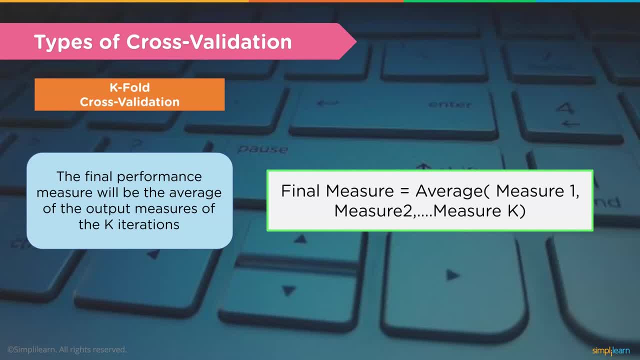 There's going to be five measurements and we'll divide that by five and that gives us a good guess, a good estimate of what the measure is on this particular cross-validation going on and how good our model is. And then you train the model with all the data in the end, because you don't want to leave one section. 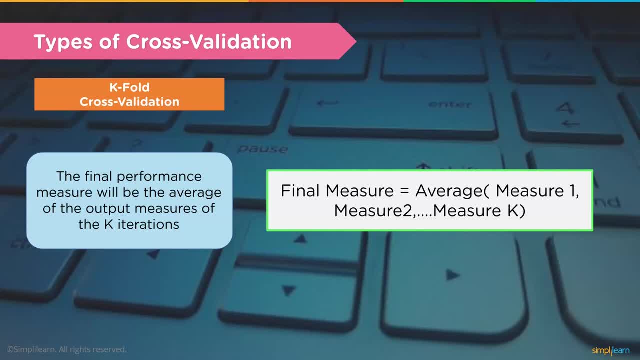 out Now one of the things- and I'm going to point that out on this page before we get into the next validation: what happens if your measurements are all over the board? You've divided into five sections. One measurement is really bad, One is really good. That means there's something going on. 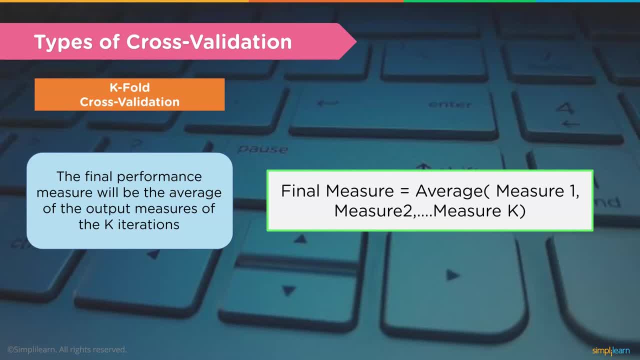 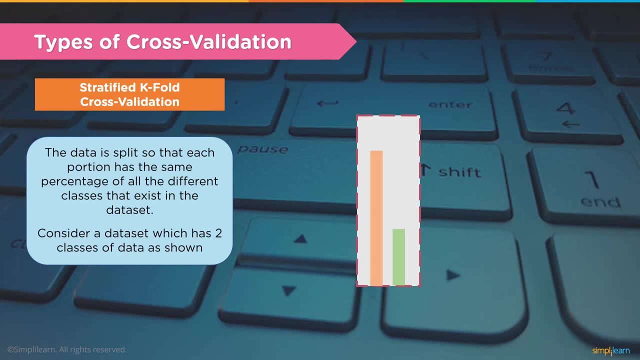 with the way you divided your data and how the data is set up, and we want to start looking at stratified k-fold cross-validation. The data is split so that each portion has the same percentage of all the different classes that exist in the data set. Consider a data set which has two classes of data. 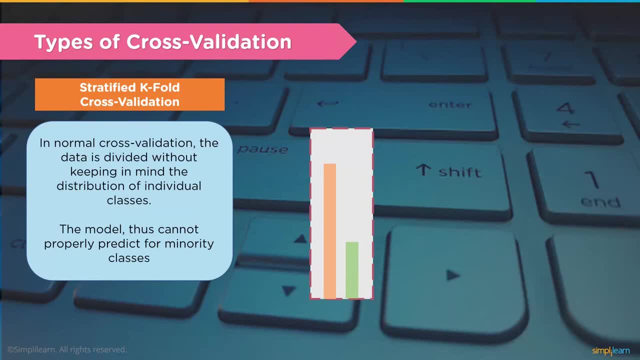 as shown In normal cross-validation, the data is divided without keeping in mind the distribution of individual classes. The model thus cannot properly predict for minority classes, And you could think of this in that if you were. let's say, you had data set that was looking at drivers. How good do drivers do when driving their car? 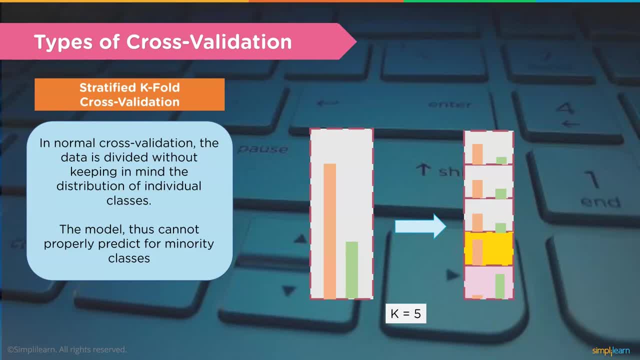 And one of the features is the color of the car. Now, my guess it probably wouldn't have a huge impact as far as the data, but let's face it: the most common car out there is probably white, there's probably brown and you get into. 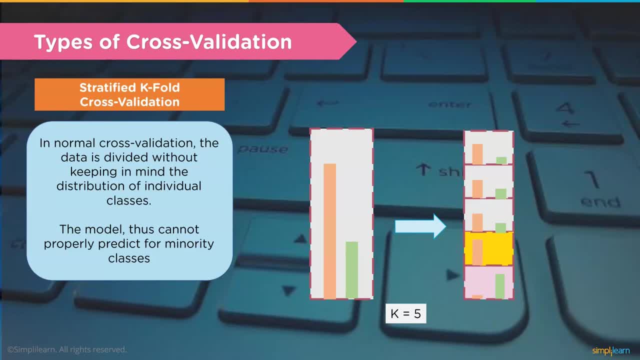 like fire engine red, It only has a few red cars. At that point, if you train your data on only cars that aren't red, you're going to run into a problem when the red car comes up, because it might have one model that says red cars are bad drivers. 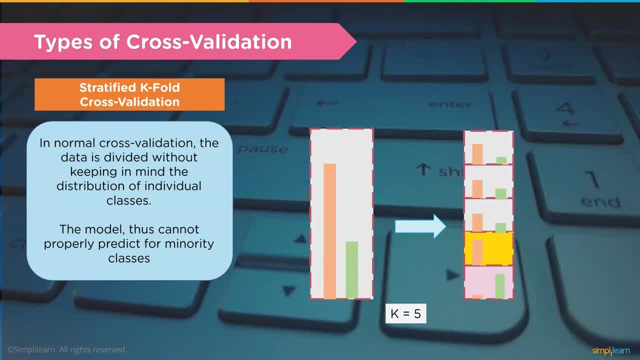 or one model that says red cars are good drivers, And at that point it's going to weigh the data and create a bias. So you need to divide up all those different features. This comes out extremely heavily in doing population statistics, where we might pull an area out, run the statistics, but because we're basing our statistics just on that area and the people. 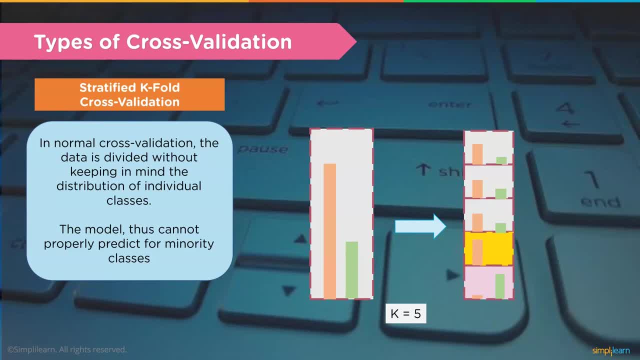 that live in there. that area might be predominantly one group of people And then you have a minority that is part of that group, but there's a bias as far as how they fit into the data and how it weighs their particular choices. And then you start running into problems with the bias on there. 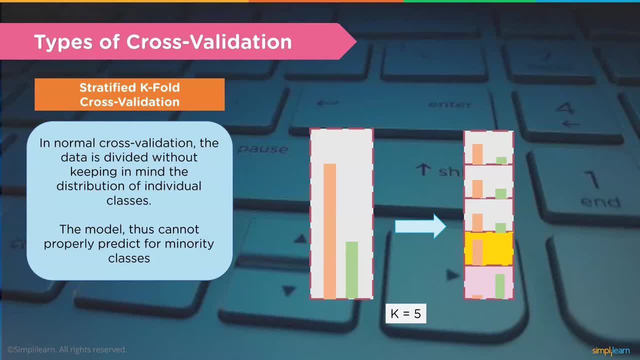 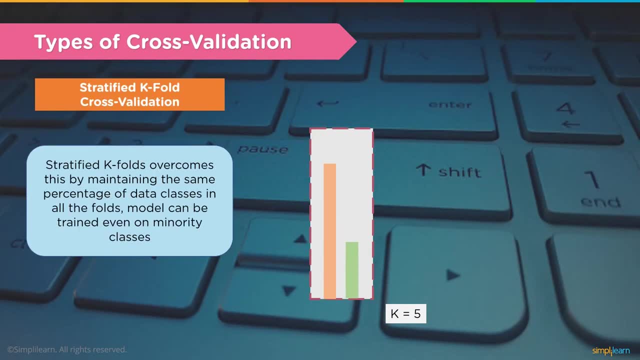 That's why using stratified K-fold cross-validation is a very important thing to add into your toolkit when you start looking at the different data structures and validating your models Models. Stratified K-folds overcomes this by maintaining the same percentage of data classes in all the folds. 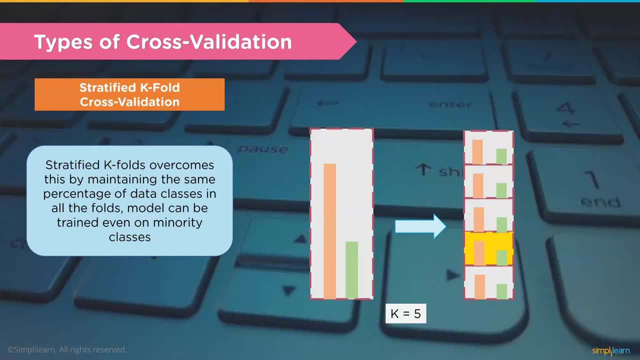 Models can be trained even on minority classes, And you can see here where, even though we have five separate splits in the data we used- K equals five- each one has a representation of all the different features in there, so that we help get rid of that bias and help each one train equally across the data. 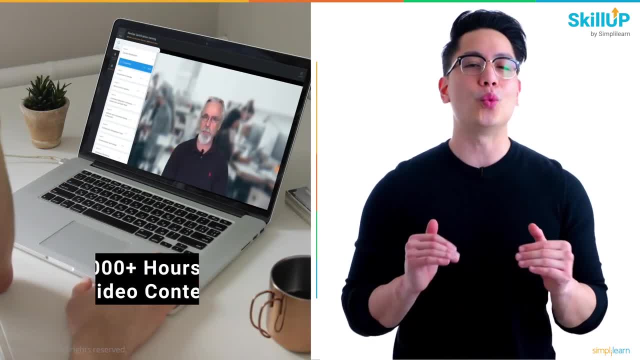 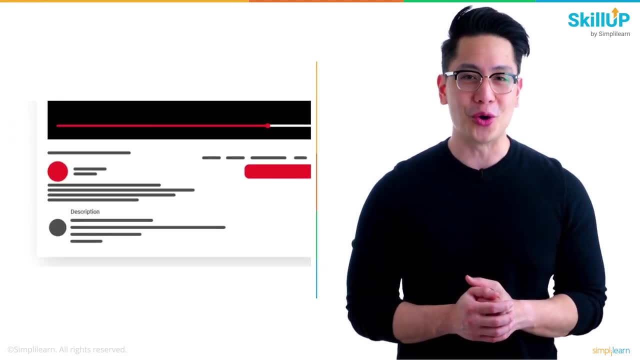 Choose from over 300 in-demand skills and get out of the box Access to 1,000 plus hours of video content for free. Visit SkillUp by SimplyLearn. Click on the link in the description to know more. So with that, let's roll up our sleeves. 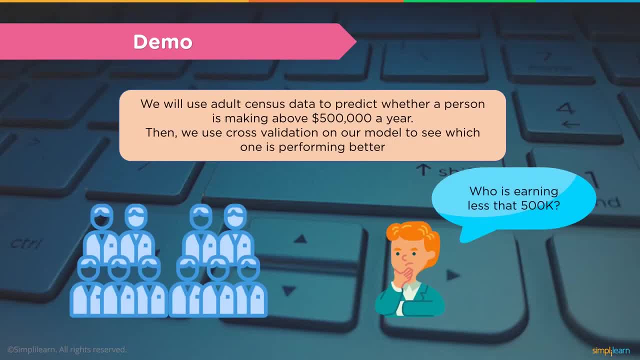 We're going to do a demo where we use adult census data to predict whether a person is making above $500,000 a year. I'm going to go out on a limb and guess that that is not US money, because that's a half a million dollars in the US. 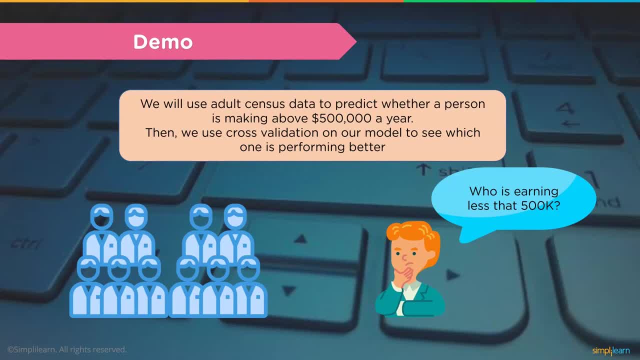 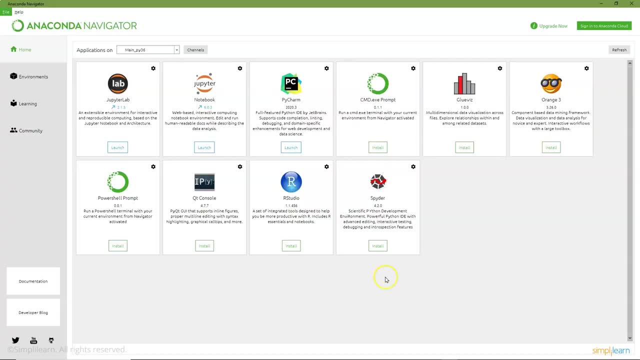 But it's still good money. Then we use cross-validation on our model. Let's see which one is performing better. Who is earning less than $500,000? That is the question we're going to ask here. For our demo, we're going to be using Python 3,. 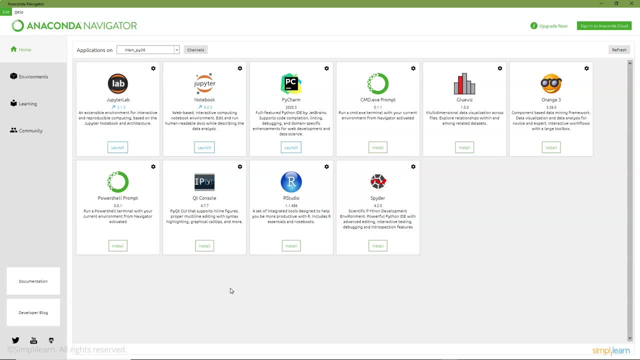 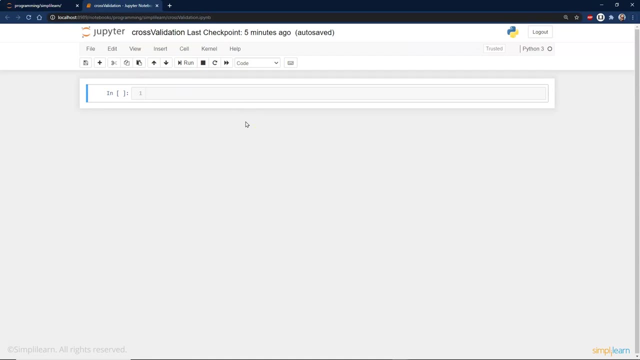 which you can use in whatever IDE you want. I myself am going to be using Anaconda Notebook, which opens up a nice web page, And from here we'll just go ahead and create ourselves a new dataset or a new Python scripting page. 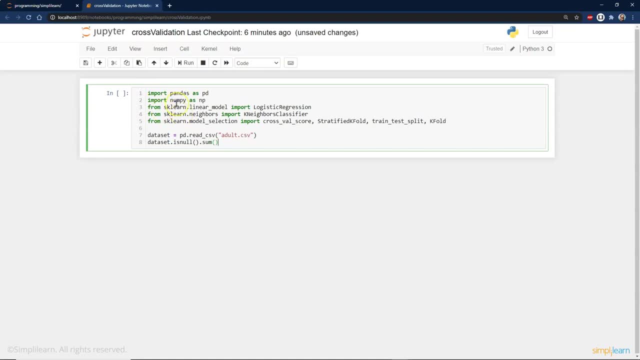 And we'll start with Python And we'll start by bringing in our different modules in here, And you'll see, in here, let me go ahead and change this to red, is fine? No, we'll go with black. We'll see, up here at the top, we have our pandas and numpy. 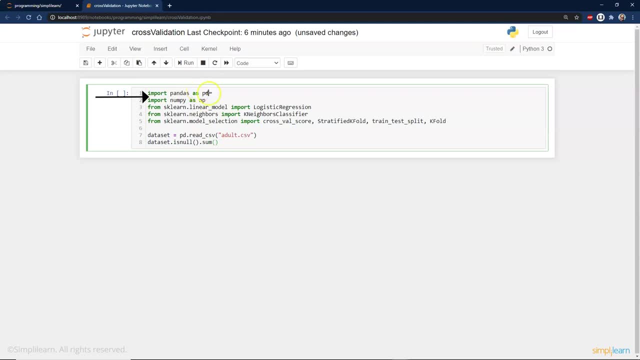 This is your numpy array and your pandas data frame, which we always like to use because they look so nice and easy to use and view. And, of course, down here, here's our data frame, here where we're going to load up our data and take a look at it. 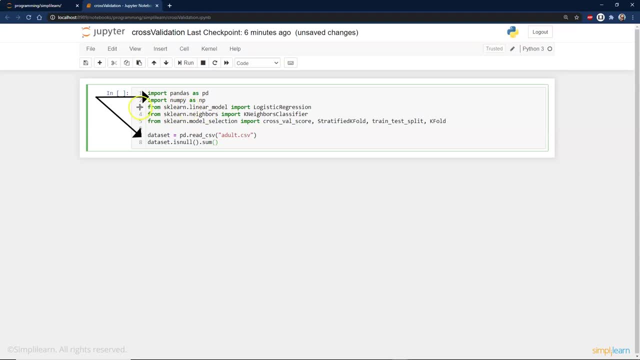 in just a minute, And then from our sklearn module, which you can see on the next set of lines. here we have our logistic regression model k-neighbors classifier and then our cross val score stratified fold, k-fold, train test split and k-fold. 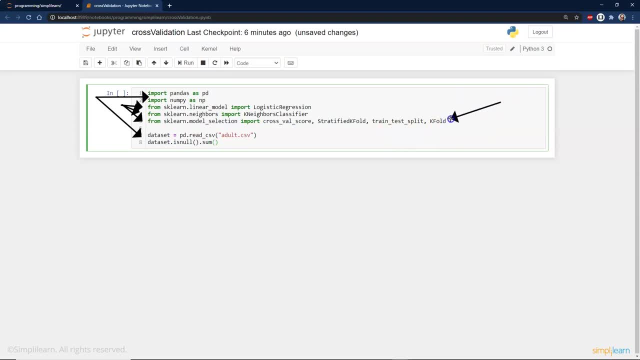 And so this is really what we're looking at right here. We're looking at how we're going to do this, We're looking at how to validate our different models, And it looks like we're going to be doing this in logistic regression and k-neighbors classifier, so we can have something to compare on there. 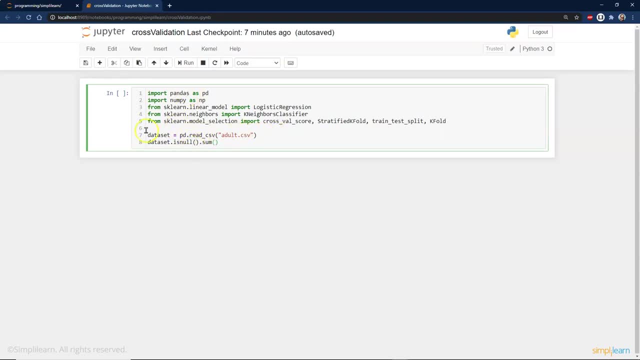 And then, of course, once we have done this, we need to go ahead and have some data. So we'll go ahead and run this. Here's our data set, And this is actually. let's see, we're using pandas, so this is a data frame. 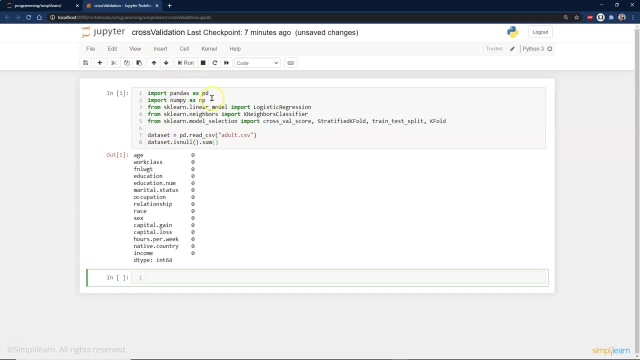 And then the first thing we're going to look to see if we have any null values. Always check your data and see what you have coming in. You just never know. And so we can see here with our quick data: set dot is null and summit. 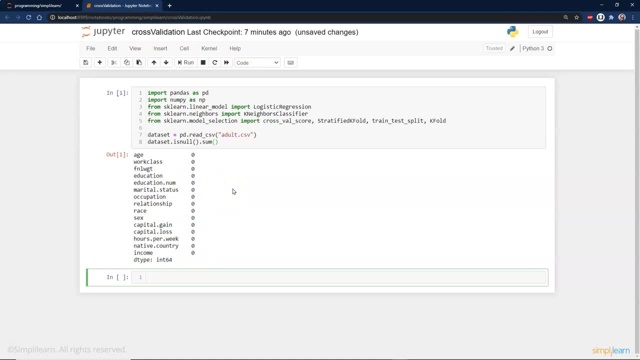 that we have zero null values in our data set. So we've read our data set in and the first step in any data is always to take a look at it. So we'll take our data set and we'll go ahead and do dot head. 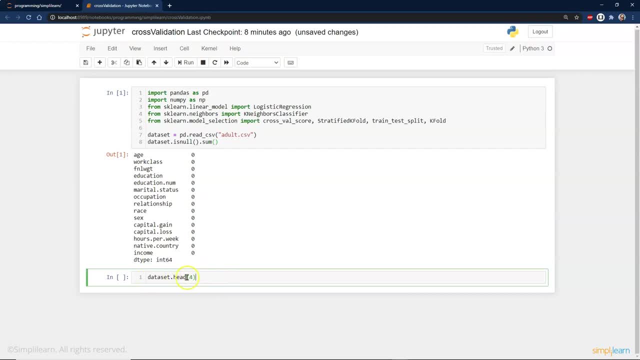 Now remember in Jupyter Notebook, if this was not the only line or the last line of my code on this particular grouping of cells, I'd have to add print around it. Otherwise it just automatically prints it for us And we can see here. here's our actual data. 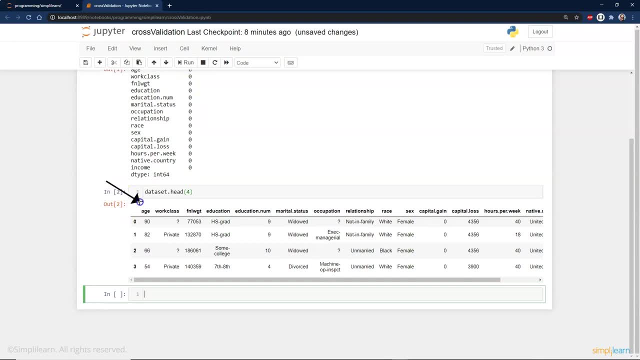 And so we have of course the titles up here: age, work class, different information, education- I guess what level of education? marital status, relationship, not in family, race, sex, capital game, capital loss, And, if you remember correctly, 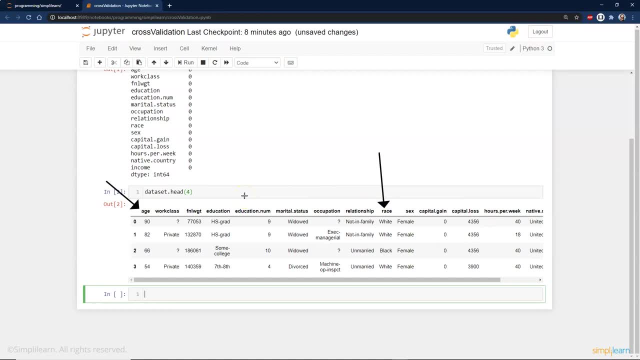 I talked a little bit about social minorities. Imagine if you were someplace where the predominant area is all in India, someplace where everybody is Indian and there's a small group of people who are what they call expatriates, who came from America and happened to be white. 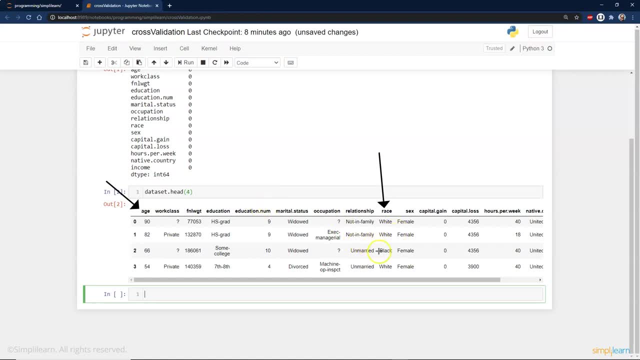 Well, you're going to run into a problem. We did that cross validation because if we're looking at this, we might notice that. or, in this case, just looking at the first four things, we see three people who are white, one person who's black, 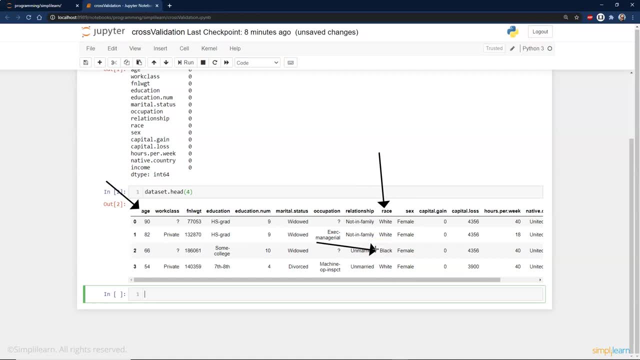 This might be a huge discrepancy in our data and we want to make sure we split that out or take a look at that. We probably won't get into that too much today, but just be aware that this is the kind of thing that you want to start flagging yourself on. 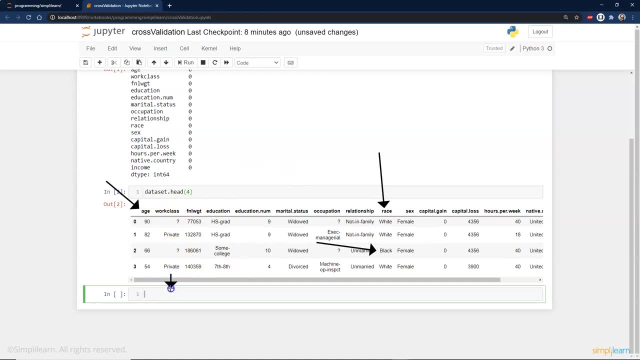 And it might be. here we have work class private. I'm not sure what that means. There's a lot of question marks here. That's kind of important to note also, And these are just some of the things I start to look at. 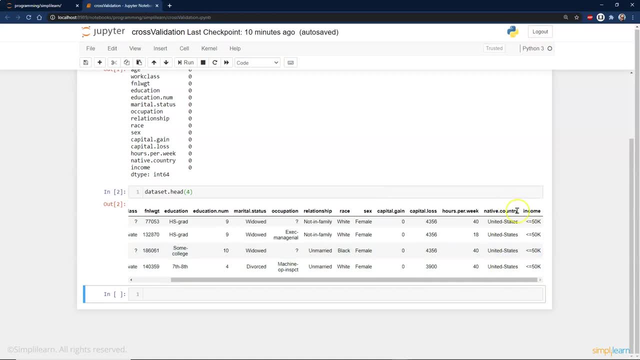 when I look at this data on here. Native country: United States. These are people coming from the United States, And here's our 50,000.. Now, remember, we're looking for 500,000.. So the average person here is probably around 50,000.. 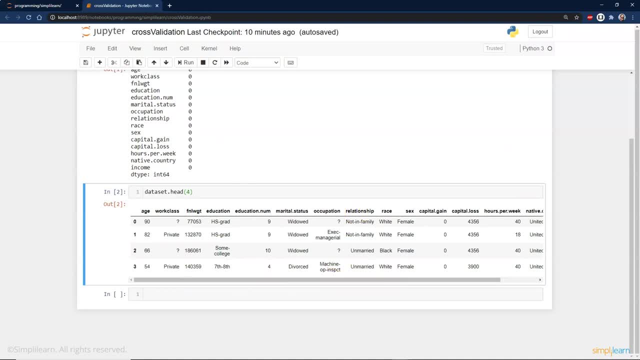 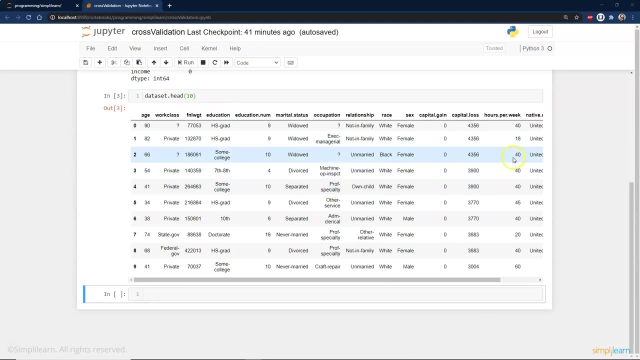 Maybe we'll take a look at that and see what kind of spread we have on our data, But it's a good place to start And we'll go ahead and do this as a print, head 10.. The reason I wanted to do that is so we could take just a little closer look. 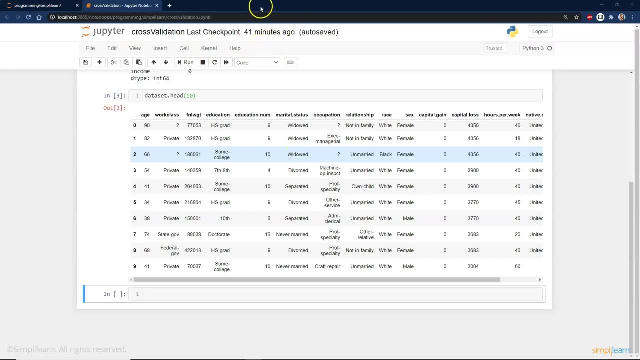 at some of the data we're looking at And if we go up here, let's put a drawing on there. Let's take a note here. under sex We're talking about that- Probably convert that to 0 and 1. And we're going to drop a lot of these columns on here. 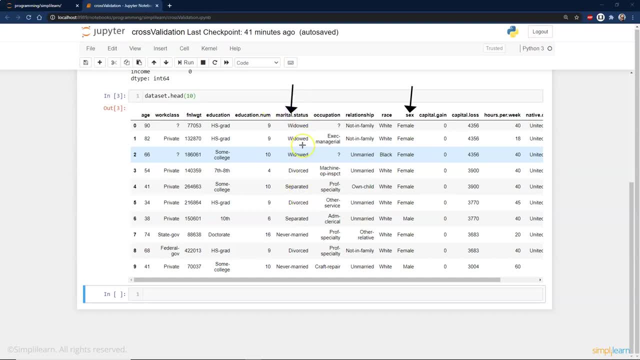 Maybe we'll also just look at marital status. We might want to convert this to 0 and 1 on here. Some other things that we're not looking at is, of course, race, And this kind of gets interesting, because when you look at race, 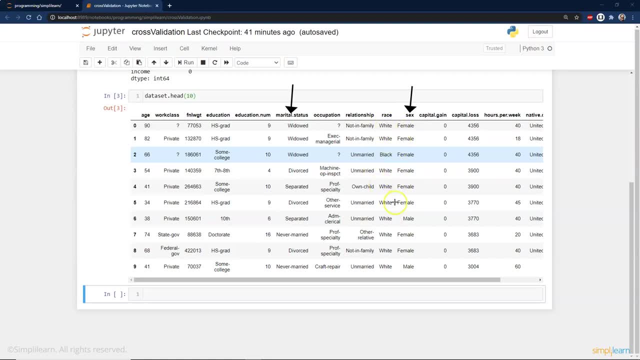 they only show right now. they only show the two variations. We'd look at how many variations there are. Same thing with male and female. If we label one of these 0 and 1,, 1 is not greater than 0.. 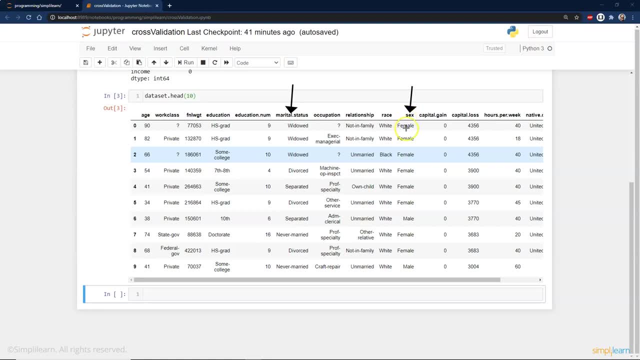 And 0 is not greater than 1.. What that means is that this is a yes-no, But as we get more variety, you can't do that. You can't do a yes-no. You have to start splitting that up into multiple columns. 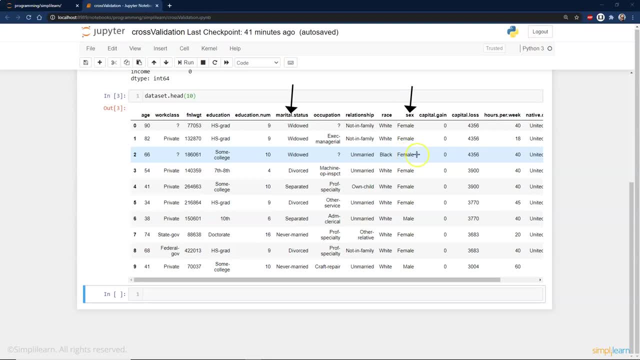 And again it depends on your data and what you find out. You might come in here. We have marital status. We'll actually look a little deeper at marital status. A couple different options in here. One is just to convert this to married or not married. 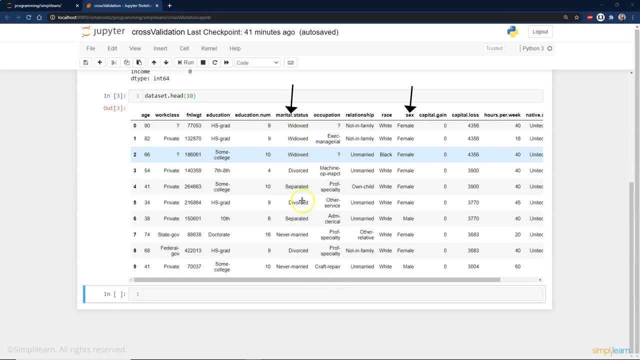 That's a 0, 1.. We might split this into columns where widow would be 0, 1, divorce would be 0, 1, separated 0, 1, and so forth. Again, it depends on what kind of data we're looking at. 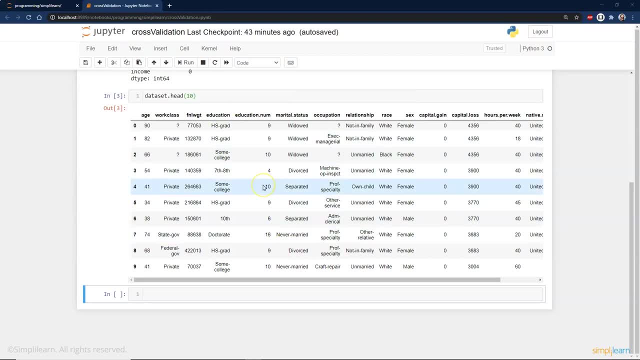 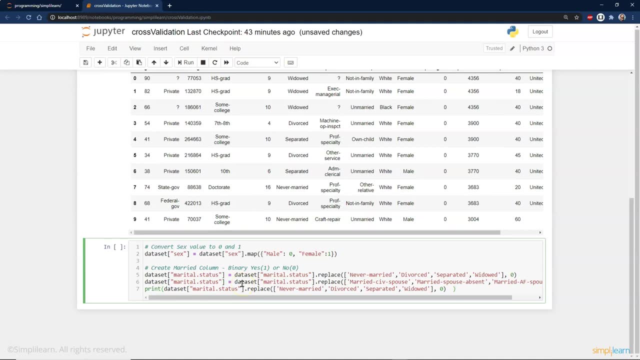 and how deep we want to get into it. So let's go ahead and clean up our data a little bit here. Let's start by cleaning up a few columns, And again we're going to drop a bunch of these Because we don't want to spend too much time cooking our data. 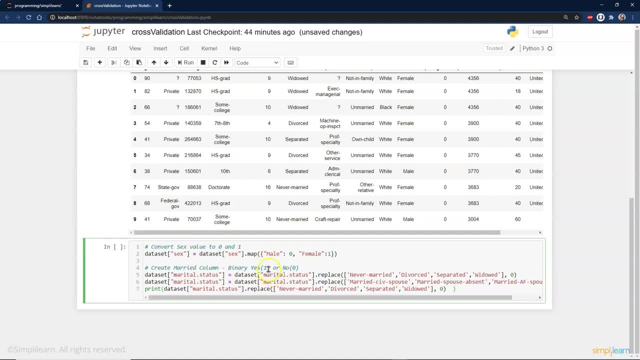 and getting it all set up correctly. We just want to have a little bit more time to focus on cross-validation And you'll see here on this we have our here. I was talking about the sex. We're going to convert that to: male 0, female 1.. 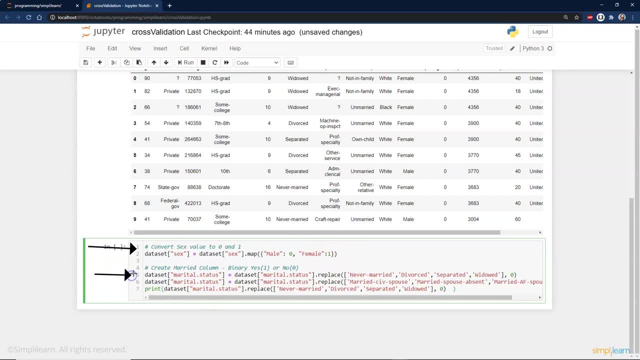 And then we'll do the same thing with married status. At this point we're going to create married status. Widow is going to- if you're never married, divorced, separated widow. it's going to be 0 for single, And then we're going to put this as 1 if you're married. 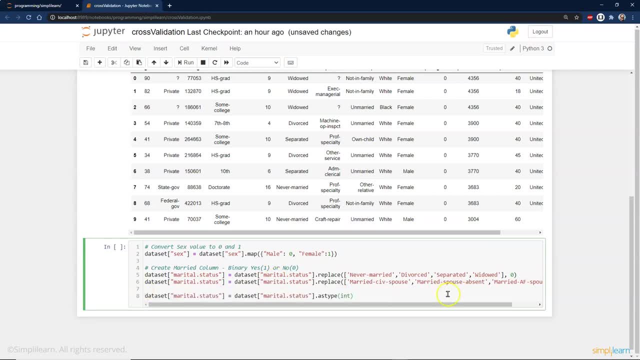 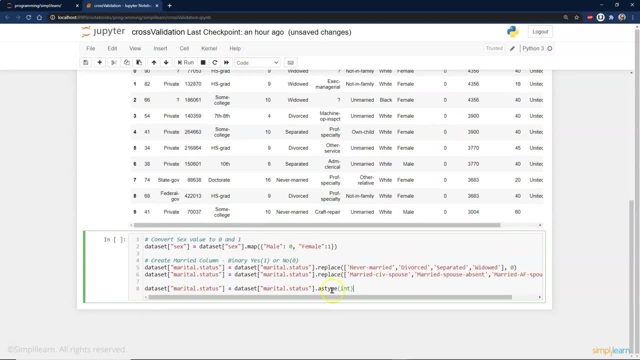 And let's go ahead and convert this into a type integer. So this works really nicely. We'll have 0 and 1 for single or married, And then there's going to be an integer. That way our different models can recognize it. 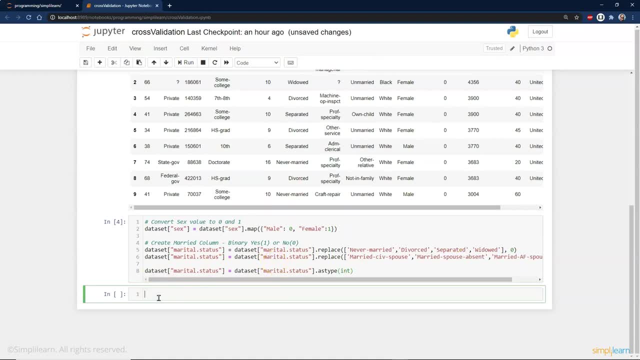 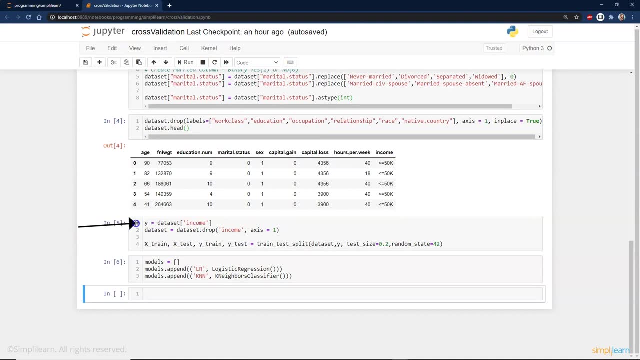 Most models don't recognize text unless you encode it somehow Just real quick. before we start looping through the different models, we've got to remember to create our y, which is going to be our income. That's our answer. And then, of course, from the data set, drop the y. 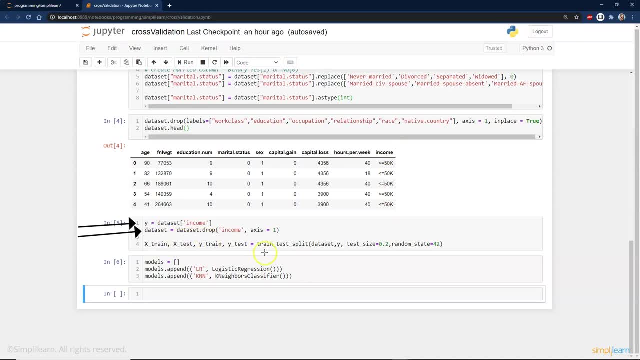 because we don't want to use it as part of the processing And the other thing we want to look at this is the code for creating our x train, y train, x test, y test. So normally a lot of times you'll see this, where we just split the data. 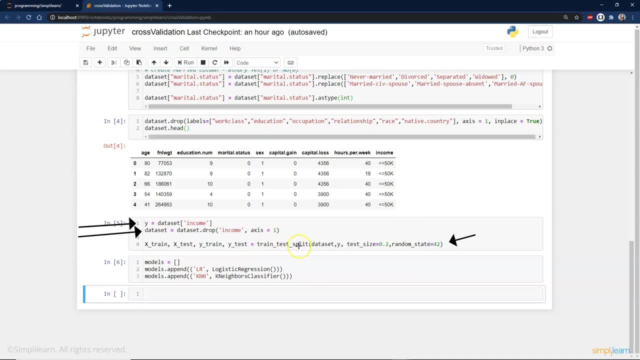 and we think, okay, good, I've got my test side, I've got my y side, But we're going to go ahead and create a loop so that we can go through this and then take a look at that as far as coming up with the results on there. 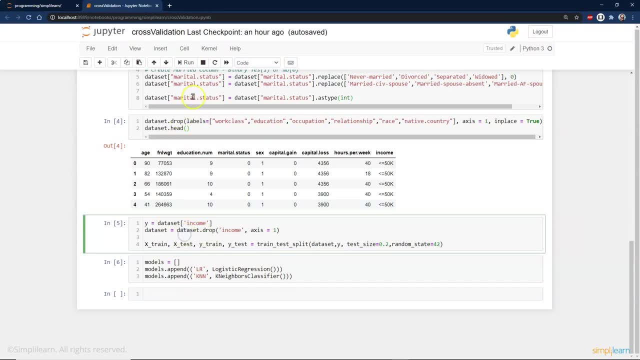 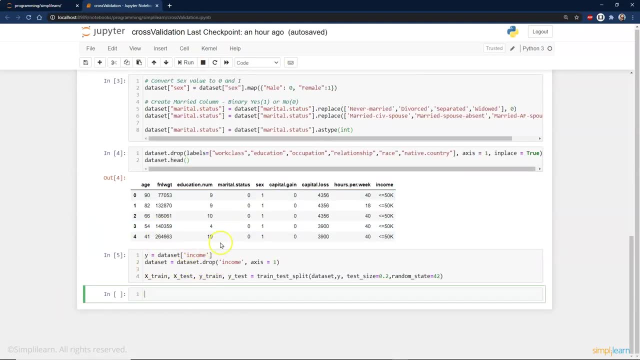 with a cross-validation score. So let's go ahead and run this And, whoops, I must have mistyped something. All I need to do is rerun the threads, because I'd run it twice and so it didn't like changing things up and I'd already run it once. 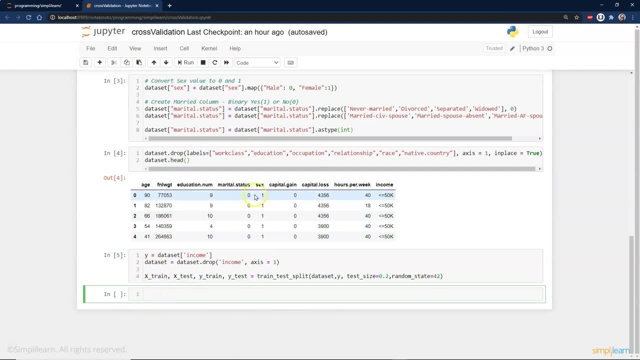 and I've already made too many changes on here, So we go ahead and run this And now we have a next step. We've got an x train and a y train. We're not actually going to do anything with this x train and y train here. 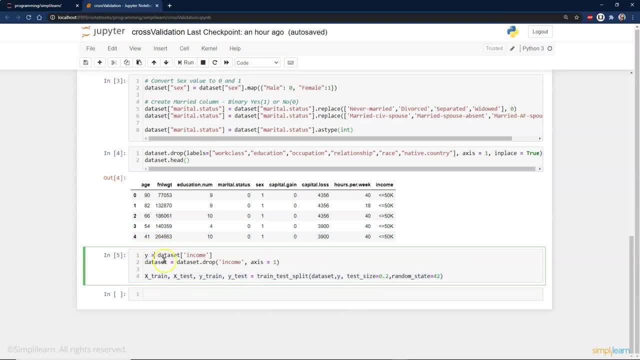 This is just a reminder for what that looks like, But we do need our data set and our y part of the data set on here. So the next step- and this is the kind of thing I love working with- is we create our models. 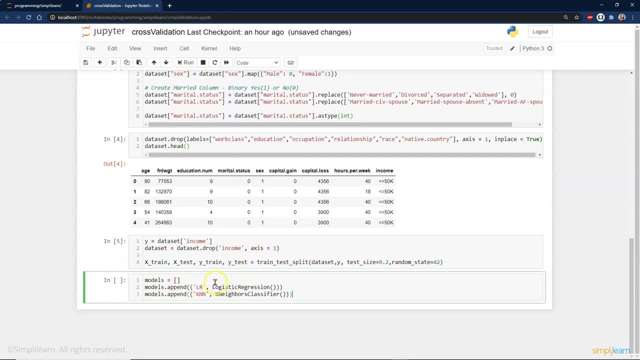 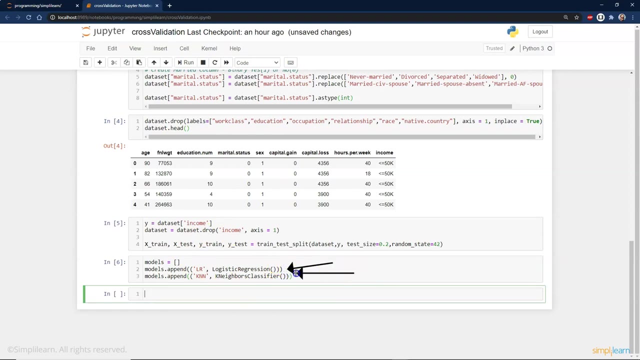 And you can see where you can start creating really robust packages to compare different models. Again, remember, this is just small data. If you did this across big data, you can run into some major problems, And so we're going to import the two different data models. 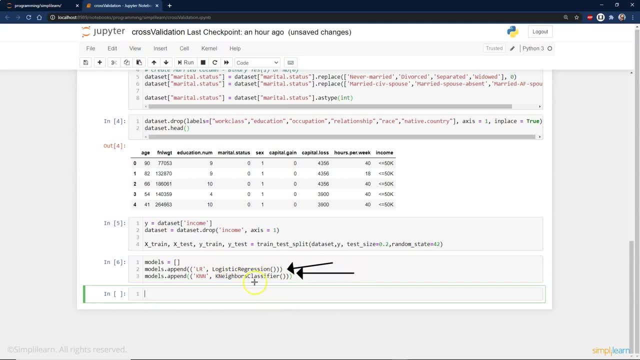 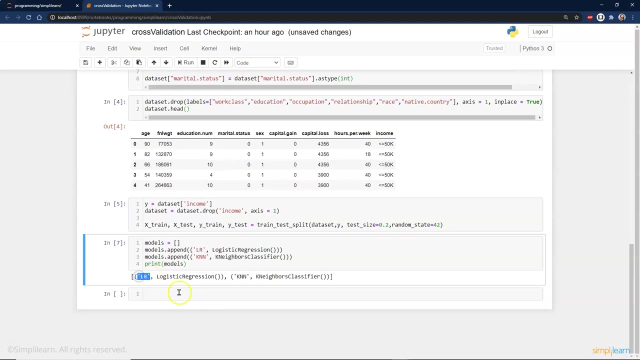 logistic regression and k-neighbors classifier And we go ahead and pin these both to models on here And if we do something like print models, we'll go ahead and run that. You can see that we have a title which is a string. 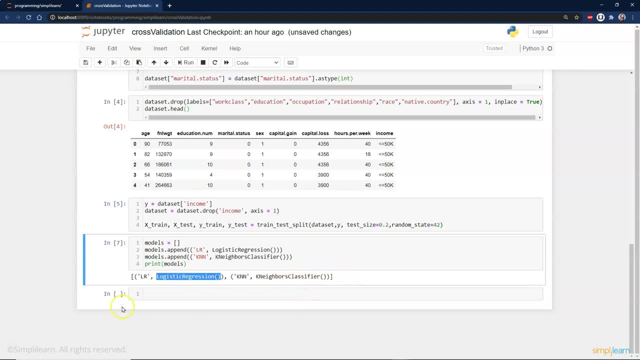 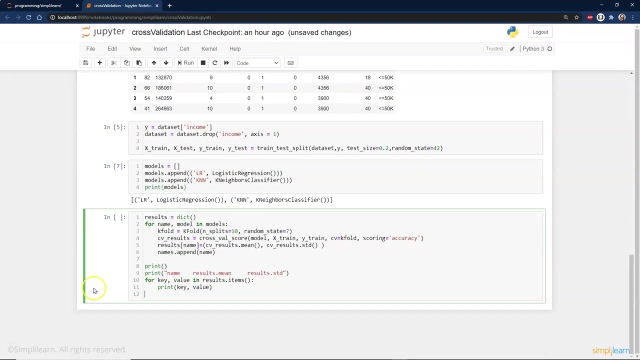 and then a function, And we can run each of these functions going through our different setup. And then what we really want to do is we want to create a loop for the different models and go through the cross validation score on the different models, And we'll go ahead and do. I'm going to create a results dictionary. 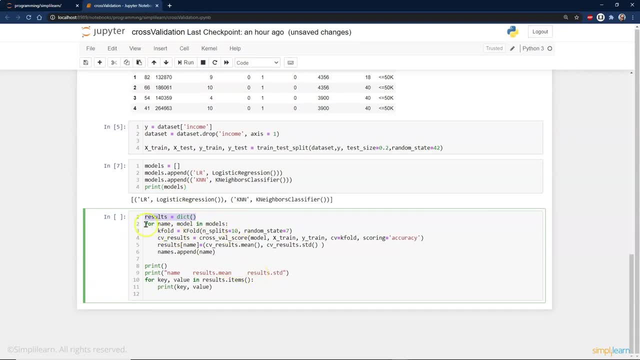 One of my favorite things to do is put everything in dictionaries And we're going to go for name and model in models. So for each row we have the name LR and then the model, so logistic regression model, And then we'll go ahead and do our k-fold. 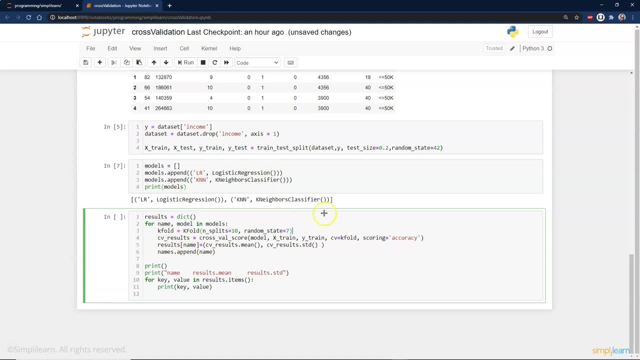 Right here. this k-fold is the heart of the setup on this. I think the random state is being changed because it threw a warning on there. and how that's being done- We'll take a look at that in just a second. the warning: 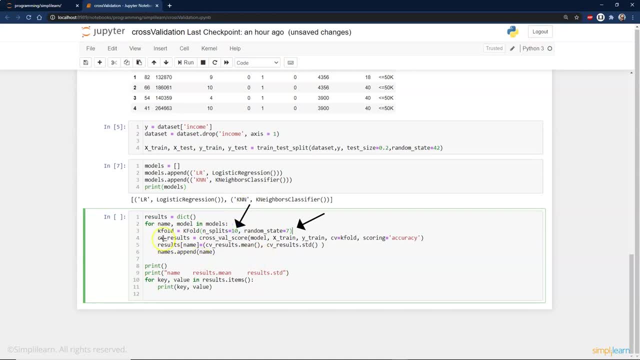 And then we have our splits. We're doing 10 splits on here with our k-fold, And then we have our results, And once we have our results, which is going to be 10, we're going to have a row of 10 pieces of data from each different fold. 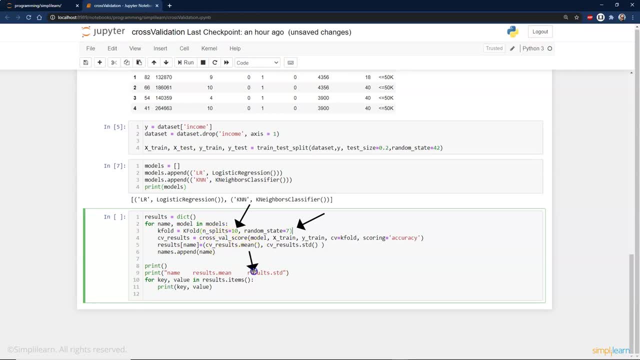 And so we want to go ahead and do the mean on that. Oops, there we go. arrow, the wrong way And the standard deviation. So how much do they deviate from each other? How low is our error on here? The lower the better. 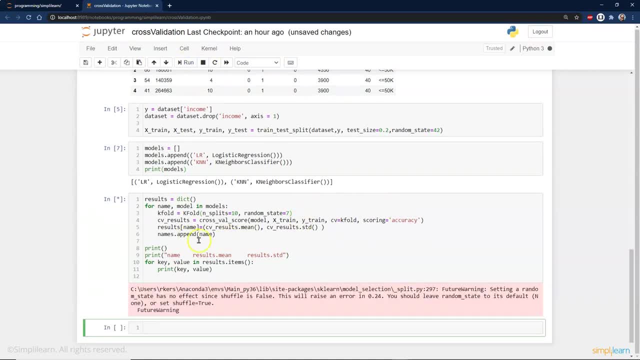 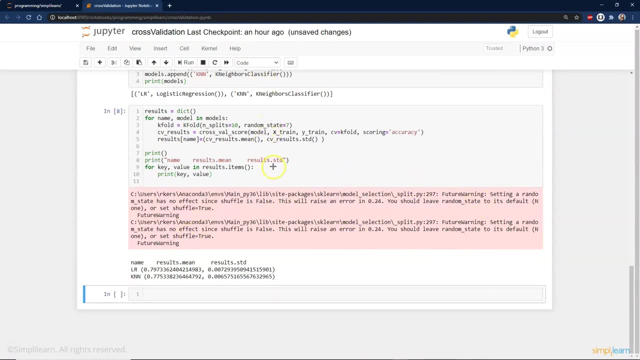 So let's go ahead and run that, And then, of course, I have on mine. there we go, we see down. here is our future warning. It says something about random states. I'm not going to worry too much about that. 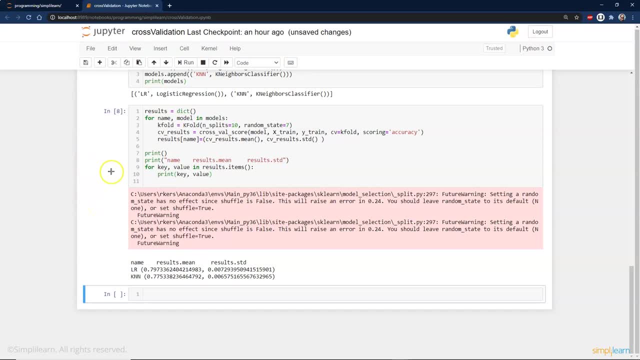 Warnings come up so often when you're running these different configurations, because they're always making changes on here, And so I've got in here my results. Here's my results with the name, And it's going to be the means and the standard deviation on here. 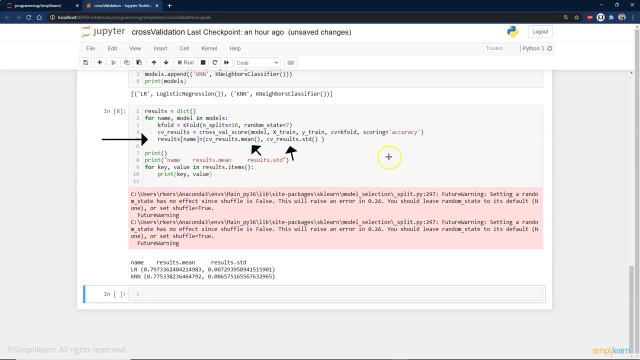 Oops, there we go that way. There's our means and standard deviation, And then I always like to do key value, just because this reminds me very much of doing mapping in larger data. You usually have a key value for your setup And we'll print the key value, which, in this case, is the name of the model. 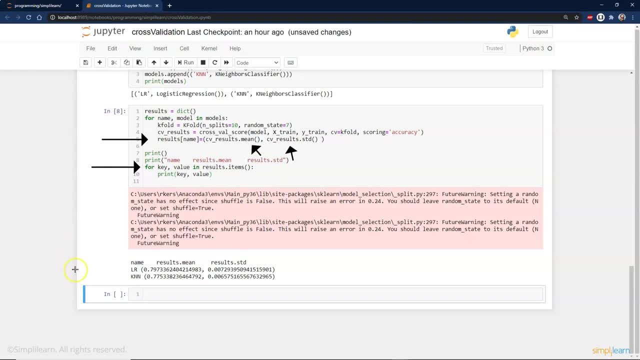 and the results on here And we can see down here. here's the two models we ran. Clearly I could add like a ton of these different models long as they are part of the sklearn setup and they use the same input. There are some models that work slightly differently. 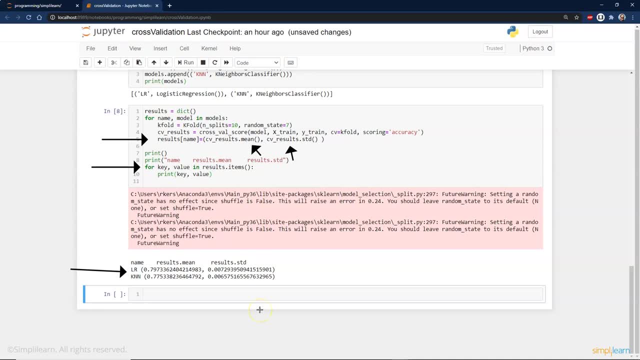 so you don't want to use. if you're doing classification and then you switch to regression, you run into problems. And of course we're doing regression here And we can see our results. the KNN did slightly better. It had lower errors. 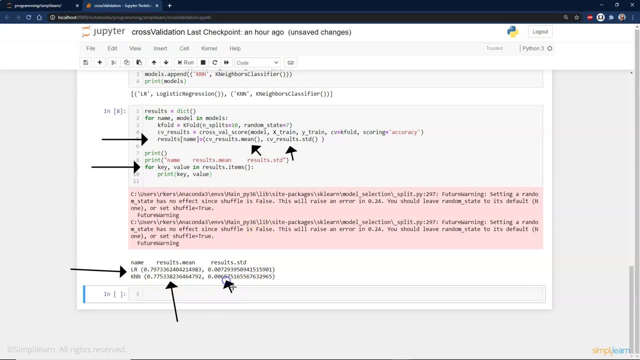 And look at the standard deviation. The standard deviation is also lower. So if I was running this model, I would go- for I'd be looking at the KNN as my primary model. I would then go rerun this model on all the data. 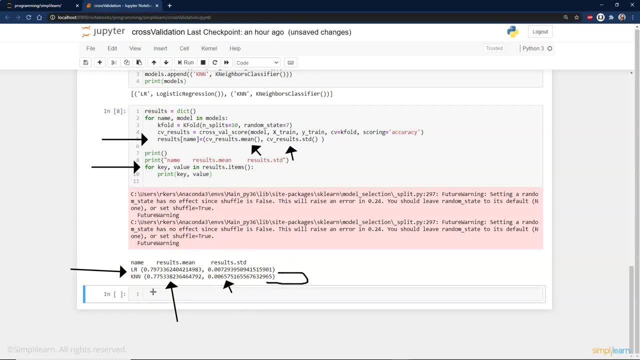 to send out for future predictions of stuff we don't know. And you can see right here: it does a nice job at 0.77 versus 0.79. And we'd pick this And you could run this across. like I said, 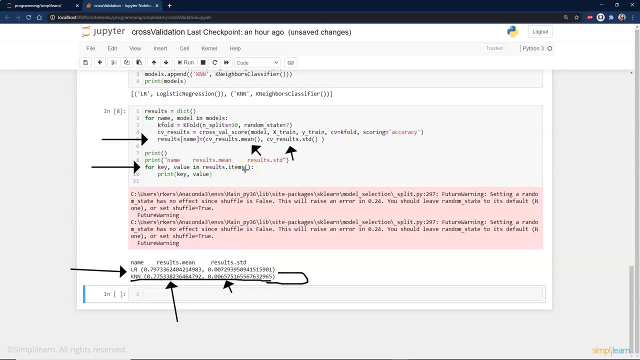 a lot of times there's like about six, seven different models in there. Some of the models have different settings, so you might go in there and mess with the settings. There's all kinds of ways to go through this, And then you can take your- in this case, cross-validation with 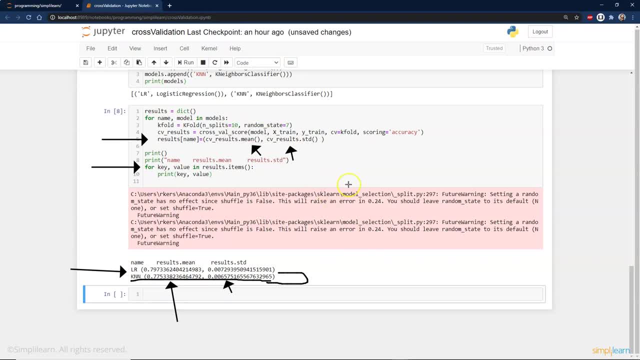 in this case, what do we have? tenfolds, And you can get a good idea of what kind of setup or which model is going to work the best And then compare it, and then you go back to your feedback loop of how to build it and send it out.